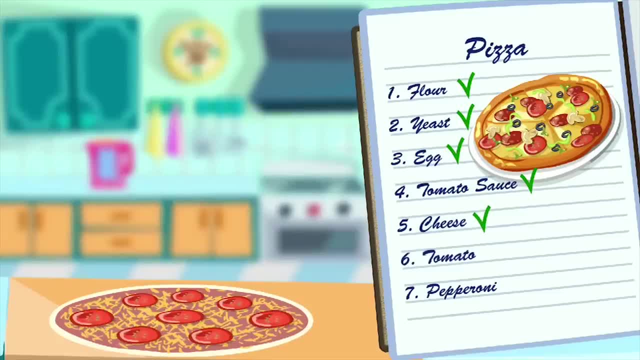 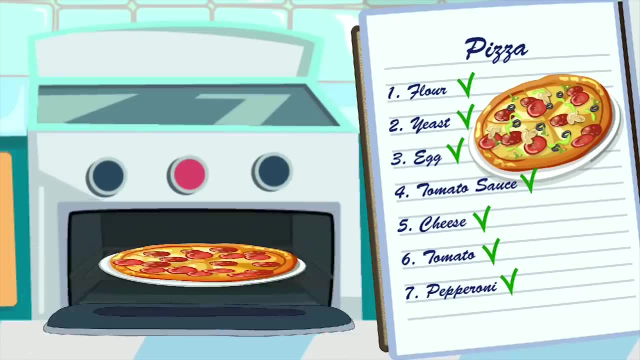 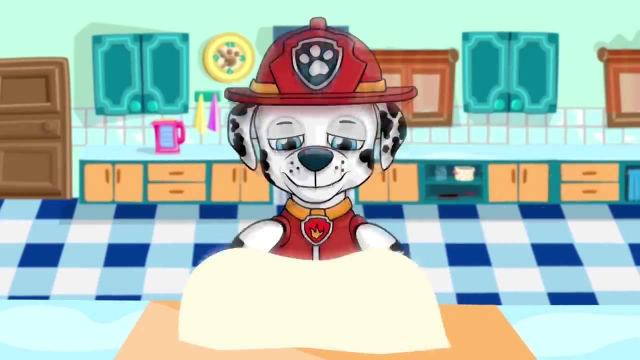 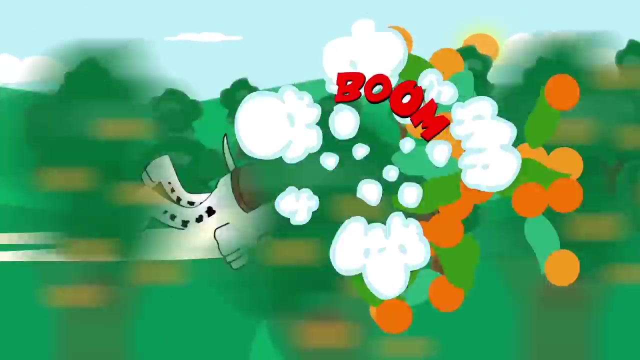 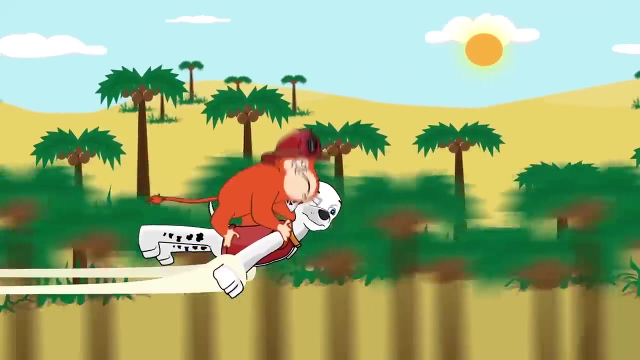 tomato sauce, some shredded cheese and tomato slices for the first, topping and pepperoni for the second. Then he'll put it in the oven for 20 minutes. Now let's see how Marshall does. That's easy. Hey, Excuse us. 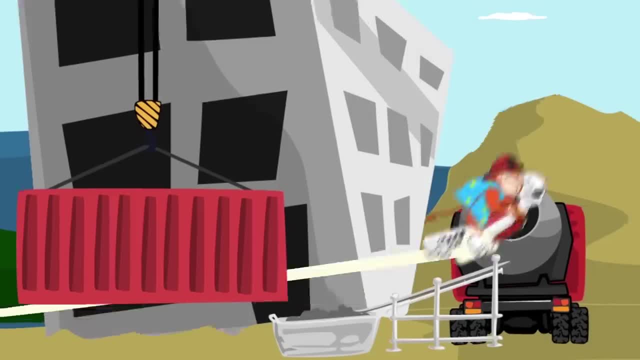 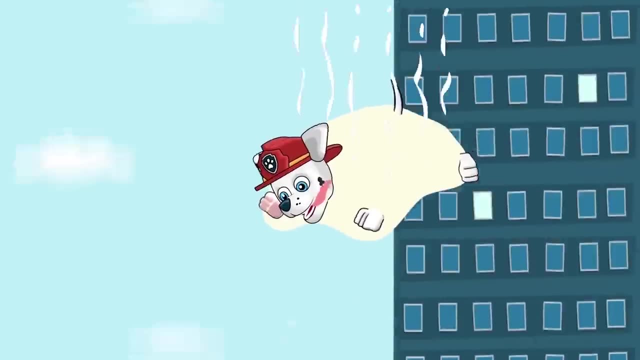 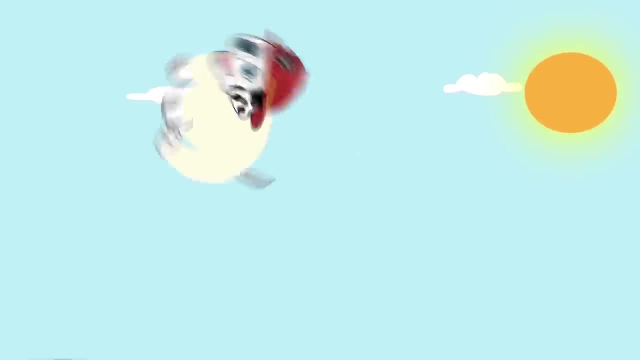 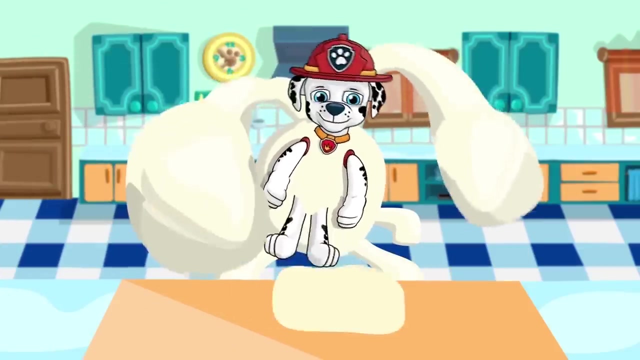 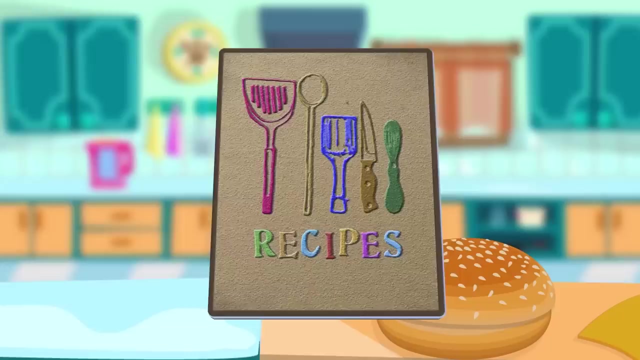 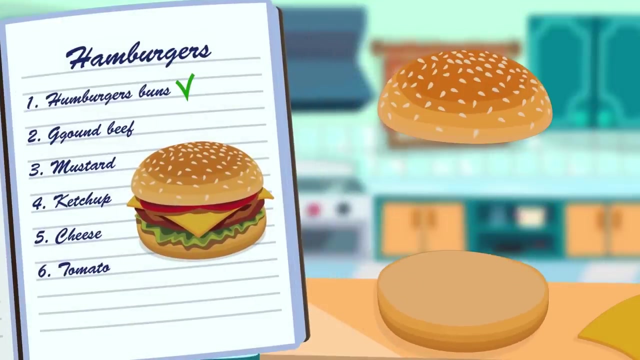 I'll take that. Just your friendly neighborhood spider pup. Now where was I? Oh right, making a pizza? Ta-da. Great job, Marshall. Let's see how Rocky handles his recipe, which is a hamburger. He'll need hamburger buns. put some ground beef in the middle, add some mustard, swirl on some. 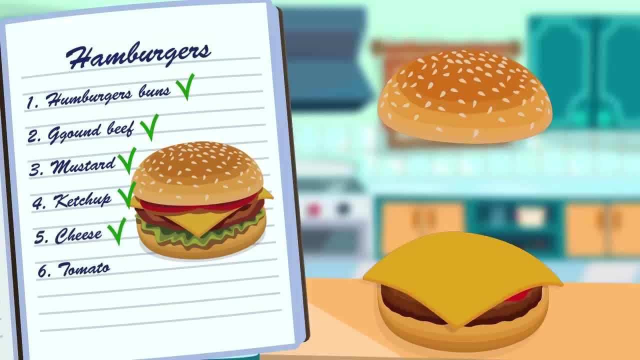 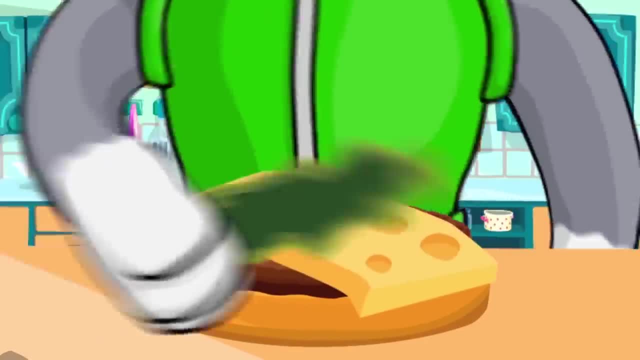 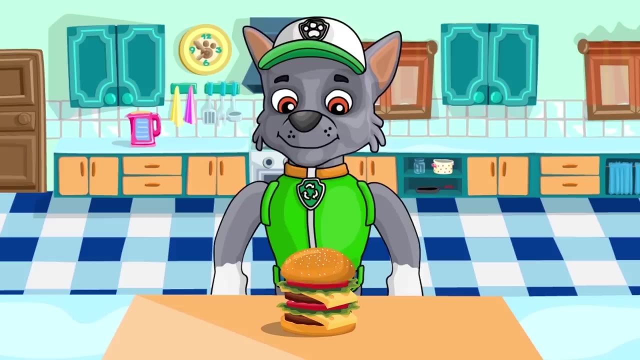 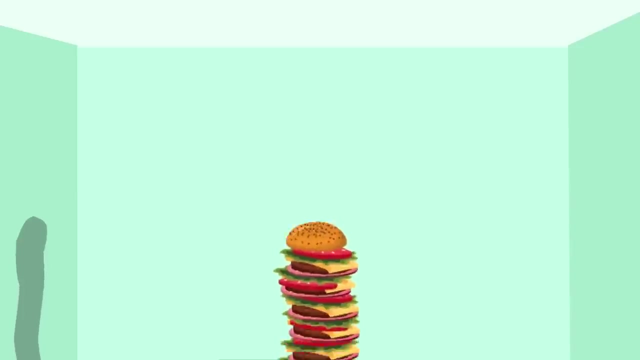 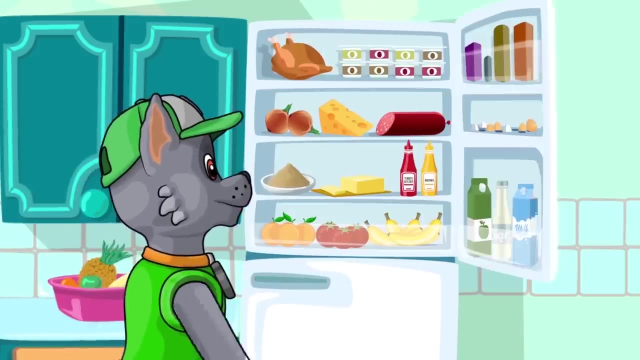 ketchup, add a slice of cheese and finally, some tomato slices. This should be no problem, Easy enough. Hmm, a little more. Hmm, just a tiny bit more. Hmm, Aha, Hmm, it could use all of these. 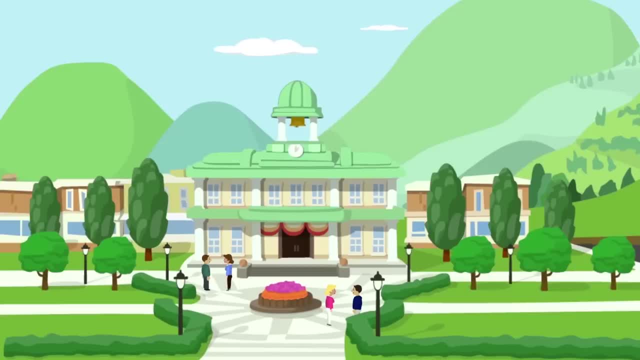 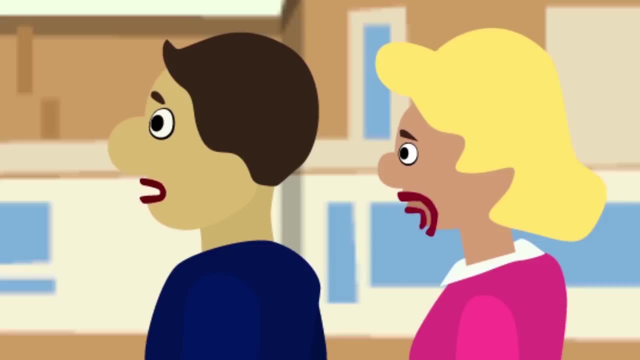 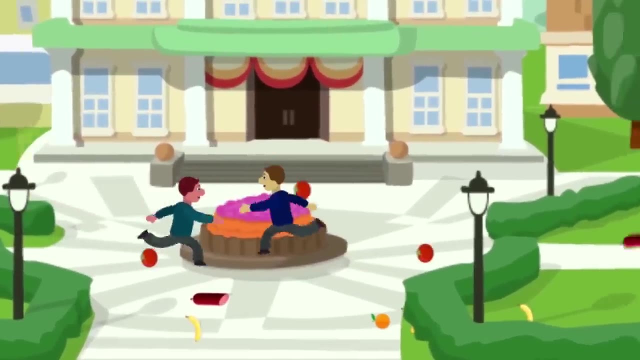 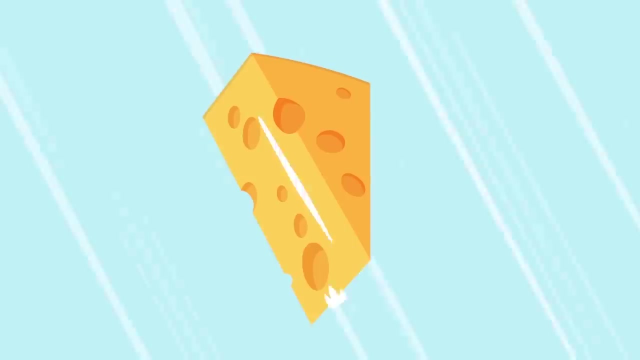 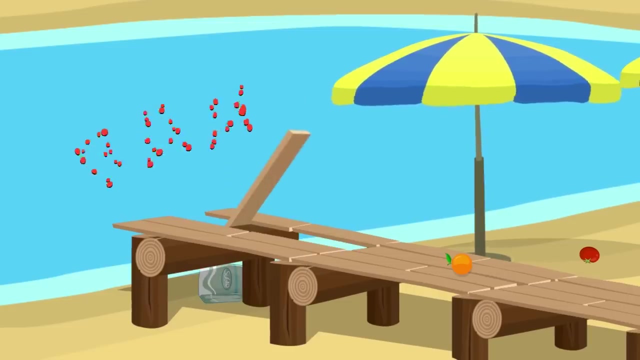 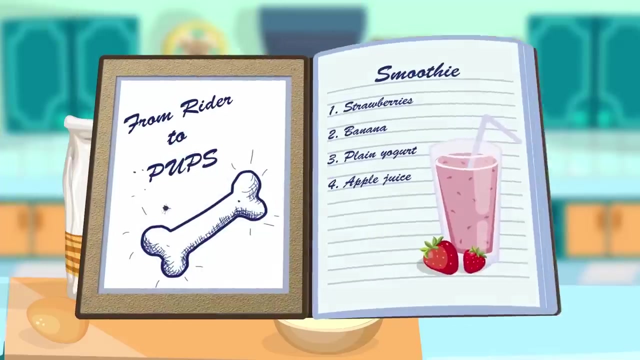 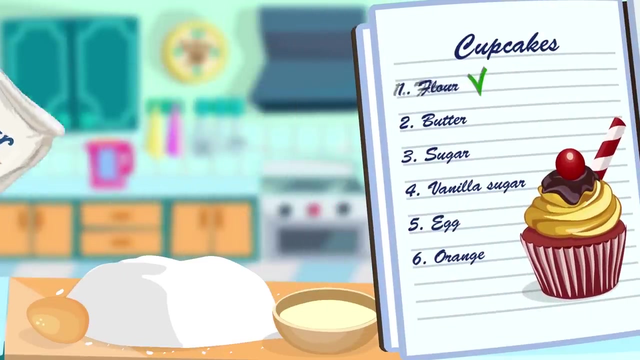 Almost almost. Oh my gosh, Oh dear, I'm running backwards. Ah, perfect, Let's check out the next recipe in our recipe book. so Skye can make some cupcakes. First you'll need some flour, a little bit of butter. 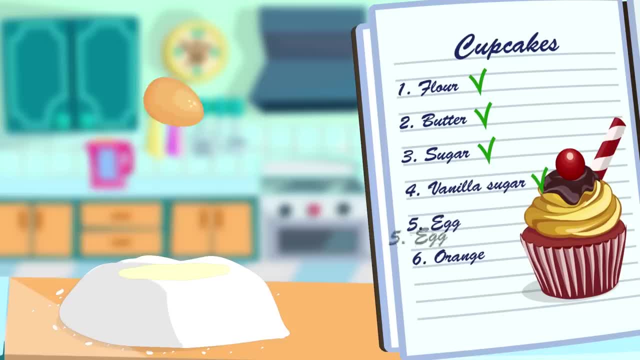 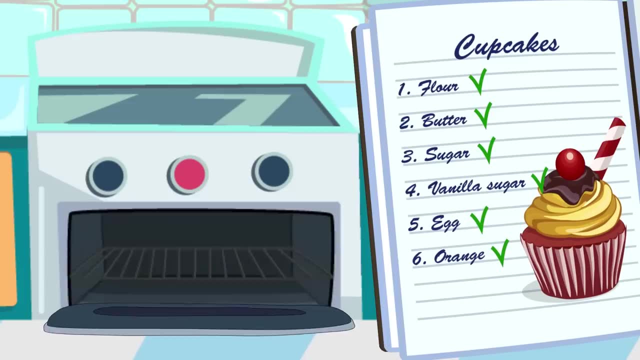 a cup of sugar, some vanilla sugar, an egg and some orange zest for flavor. Mix it all up, then put our cupcakes in the oven for 15 minutes. Alright, give it a try. Skye, This pup's got to cook. 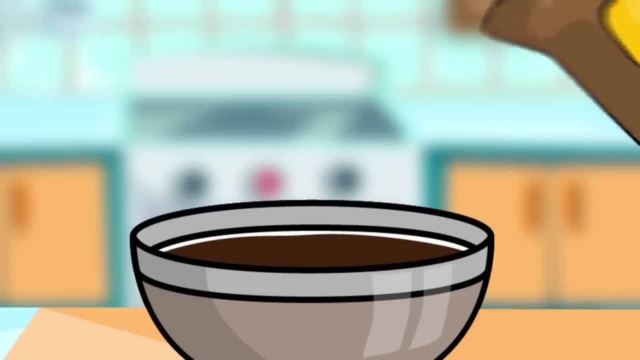 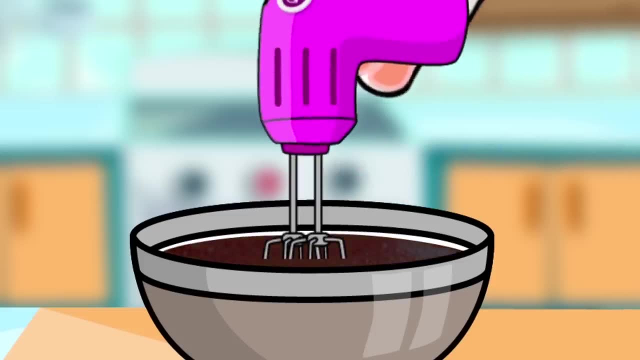 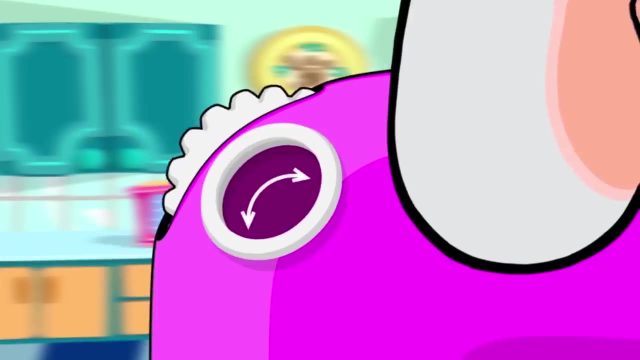 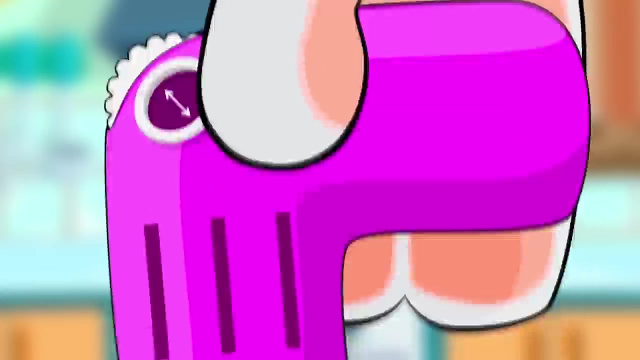 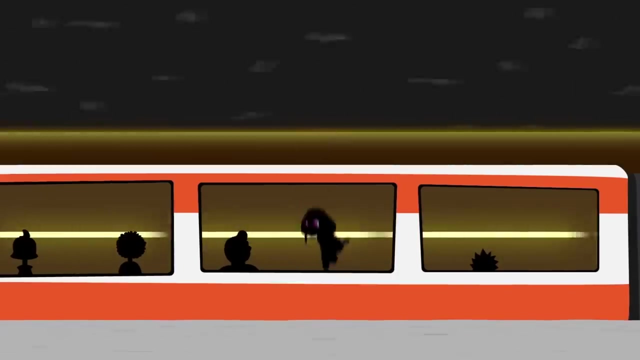 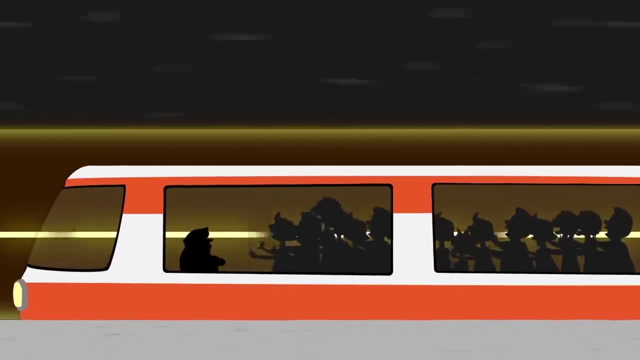 Hmm, too thin, This'll thicken it up A little more. Oh, it's stuck. Waaaaaah, Ow, ow, ow, ow, ow, Oh, I got it, I got it, I got it. 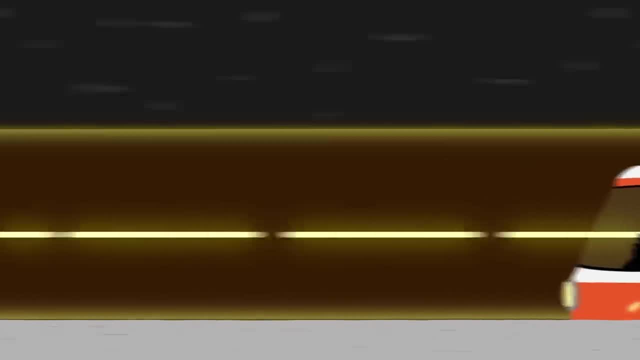 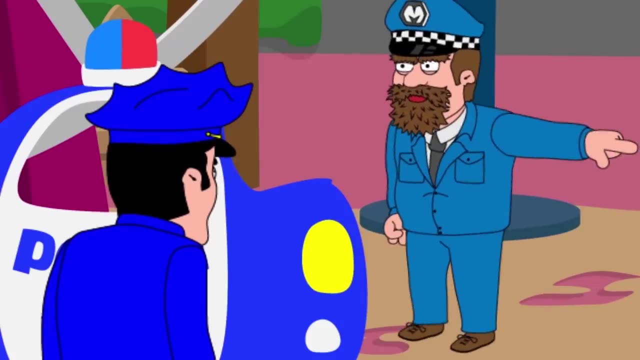 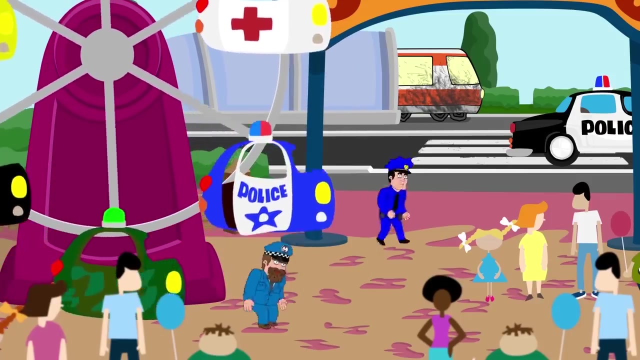 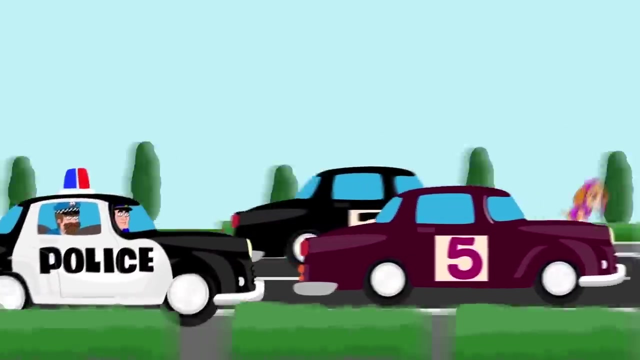 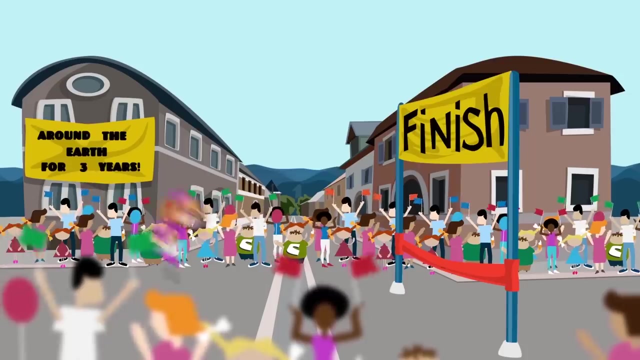 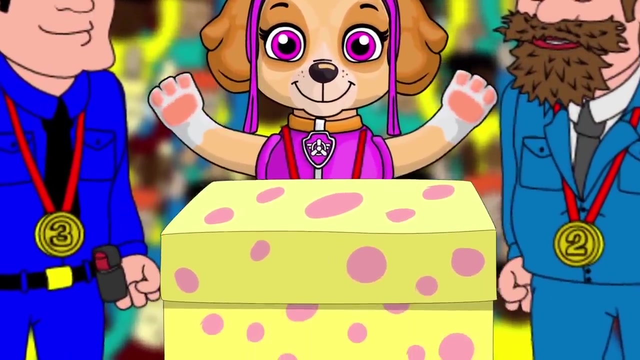 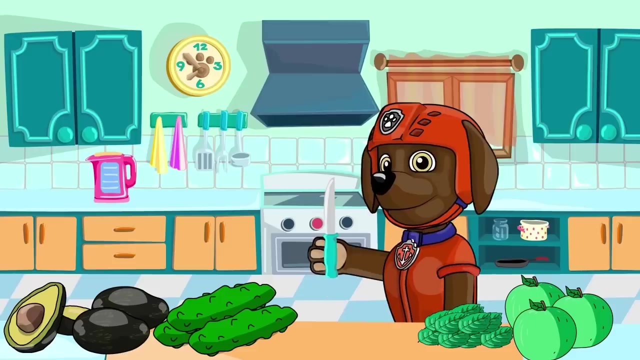 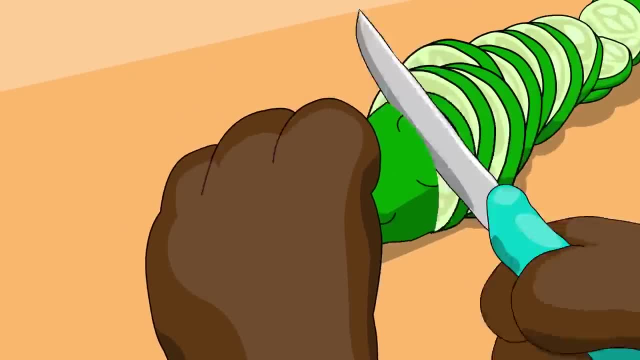 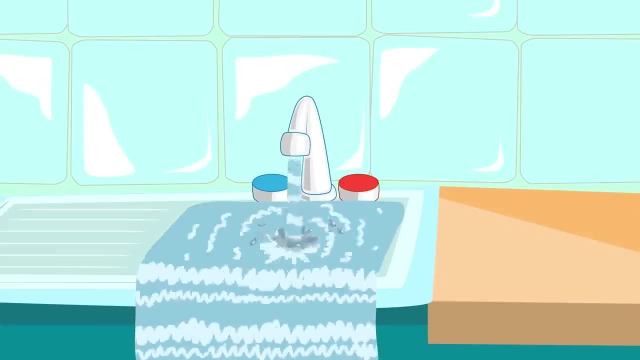 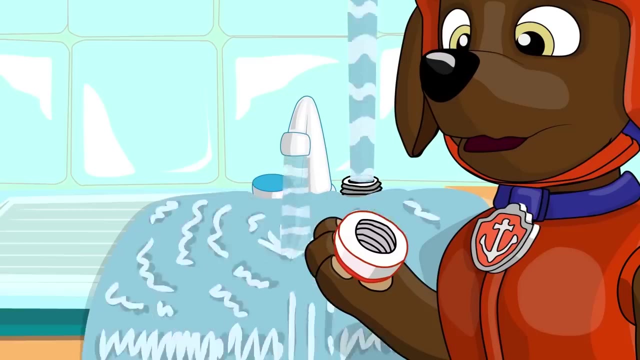 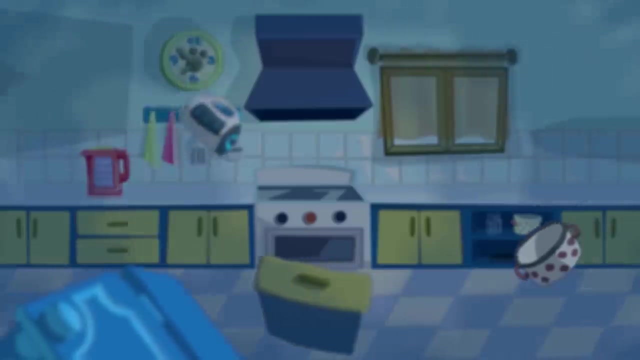 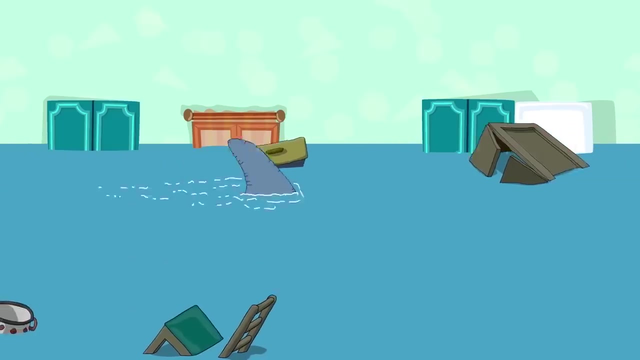 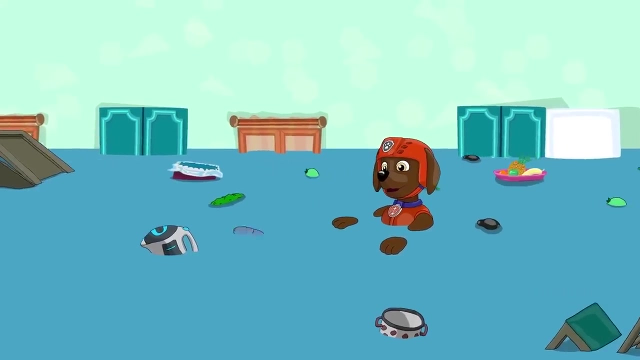 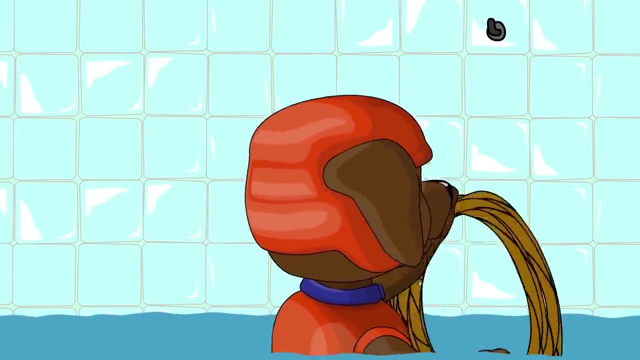 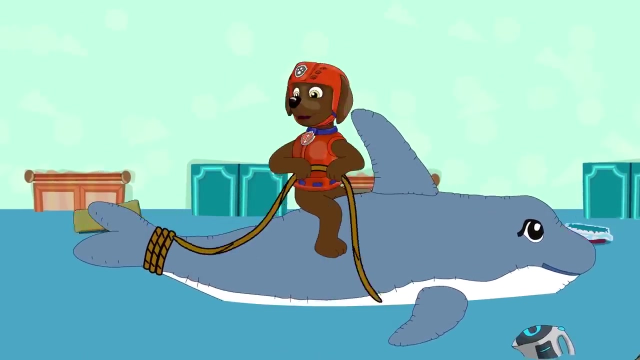 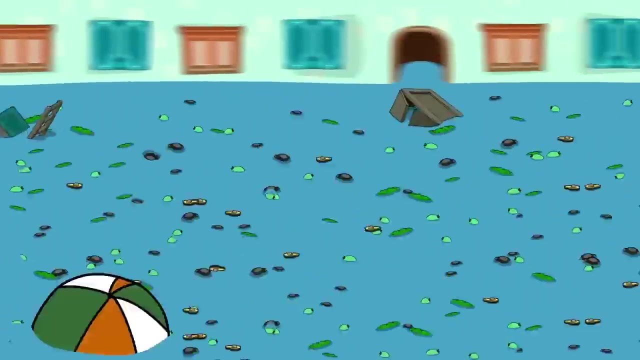 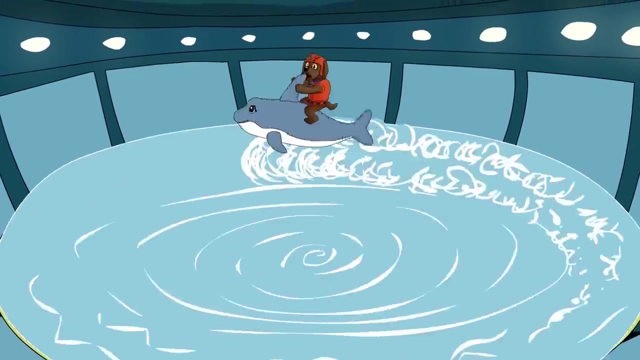 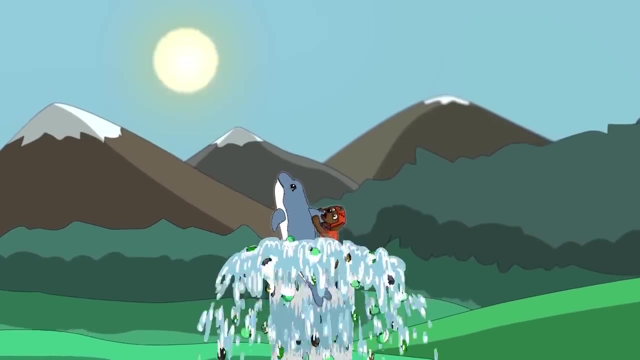 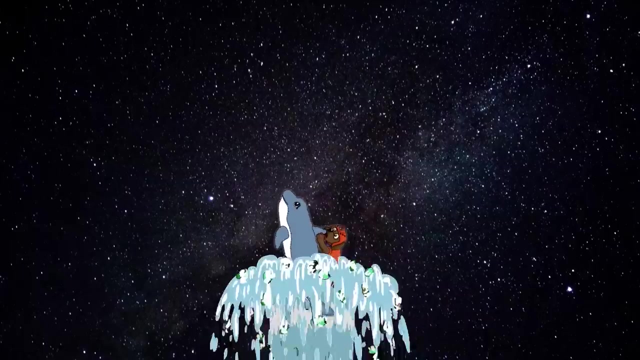 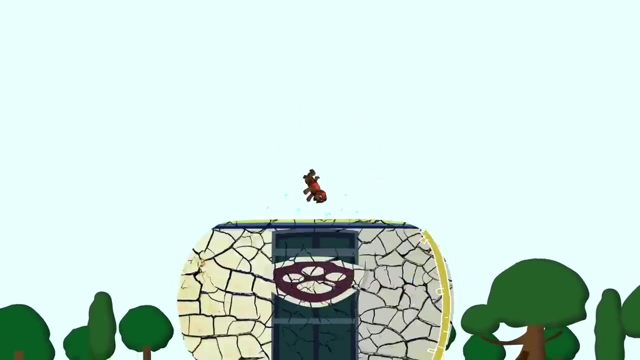 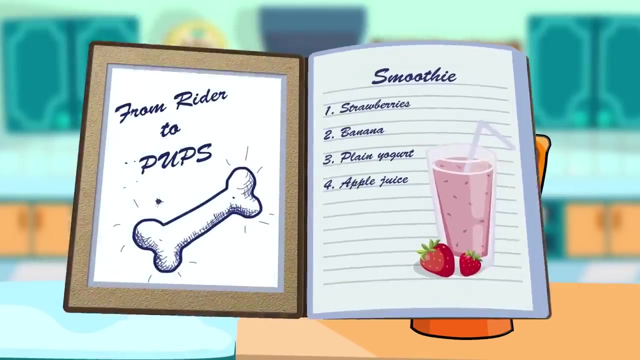 Chop, chop, chop to the cucumber. Now let's see: Oh, Baby shark, Yeah, Huh, Oh, Oh, Dolphin, Whoa, Oh, Perfect. Well, that's one way to make a smoothie, but let's check out an easier way in our recipe book and 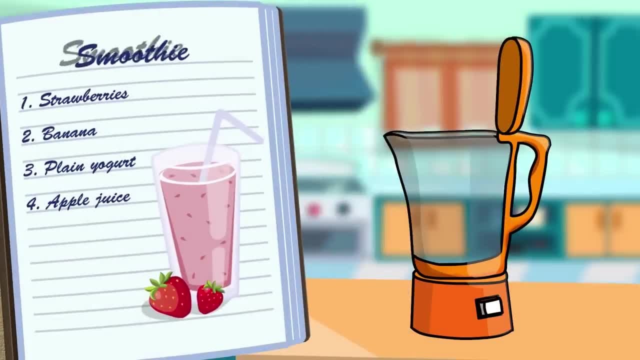 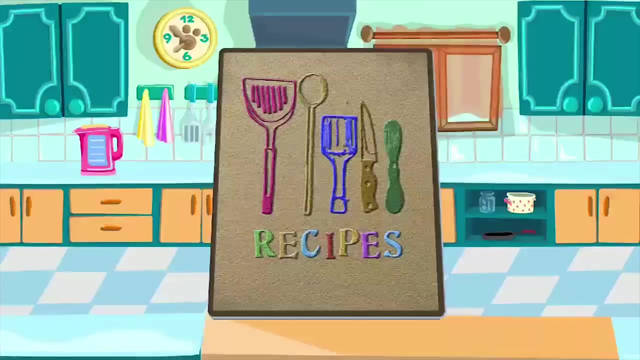 We'll add our ingredients to this blender. First we need strawberries, a banana Peeled and sliced, Some plain yogurt to thicken it up, and finally add some apple juice and Mix them all together for a healthy fruit smoothie. Now doesn't that sound delicious? Let's check our recipe book to see what Chase is gonna cook. How about spaghetti? 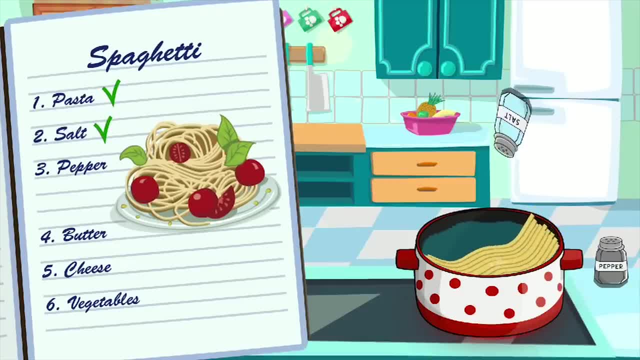 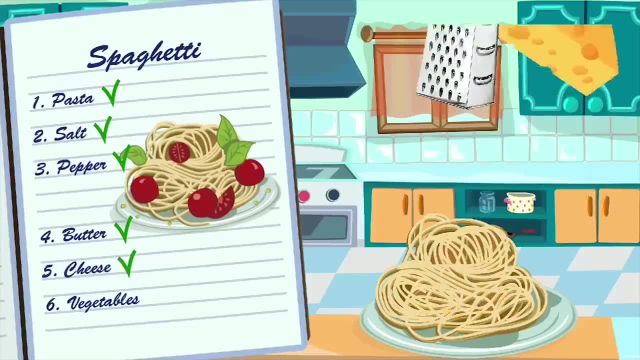 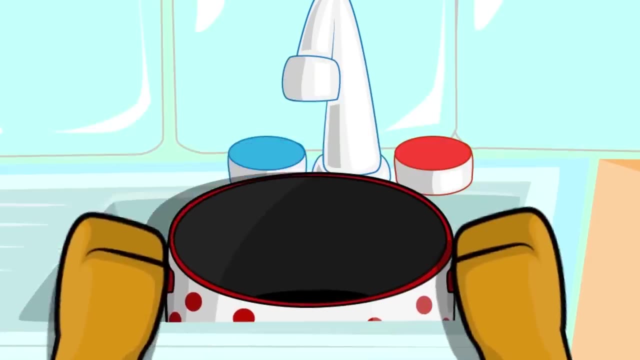 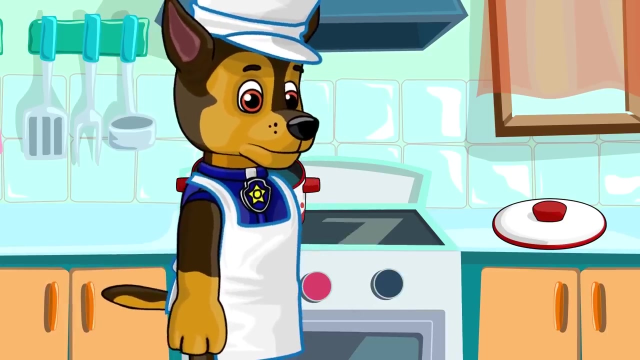 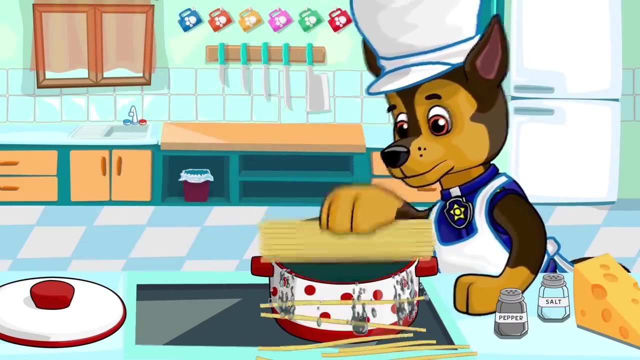 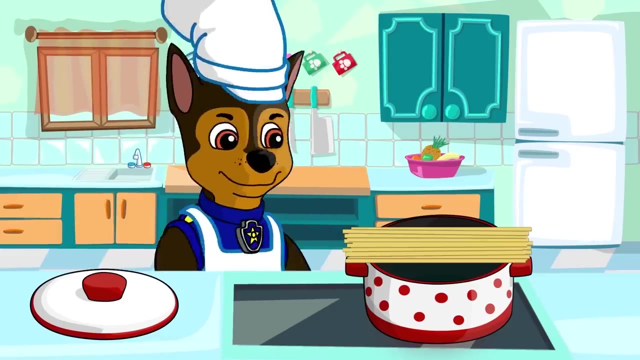 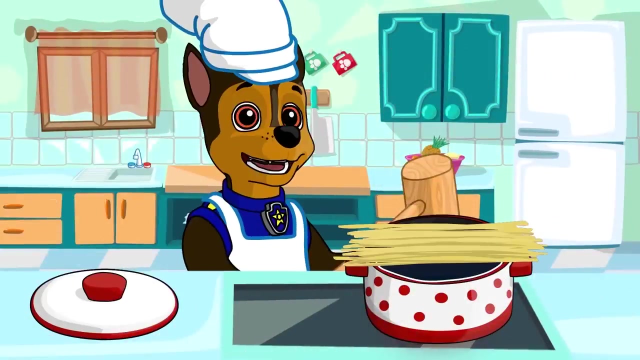 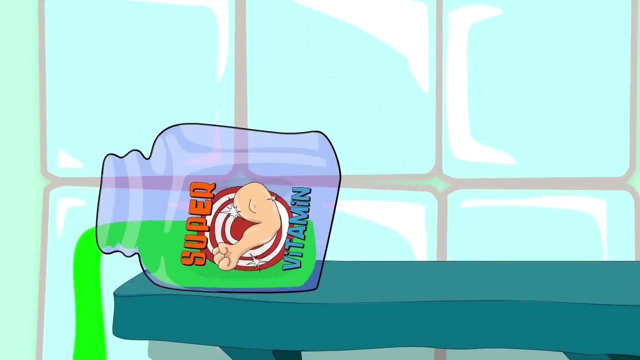 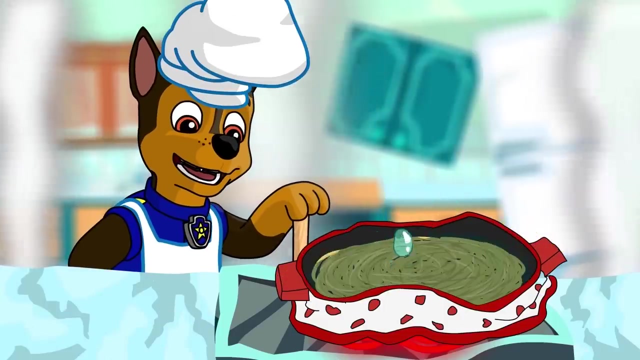 He'll need some pasta. add some salt on top and a little pepper, Some butter, grated cheese and some vegetables. It's pasta time. Hey, Whoa, Uh-huh. Okay, harder it is. Yeah, No problem, baby, We have a spare pan. Now I am gonna get it fridge and boil it for a little bit. 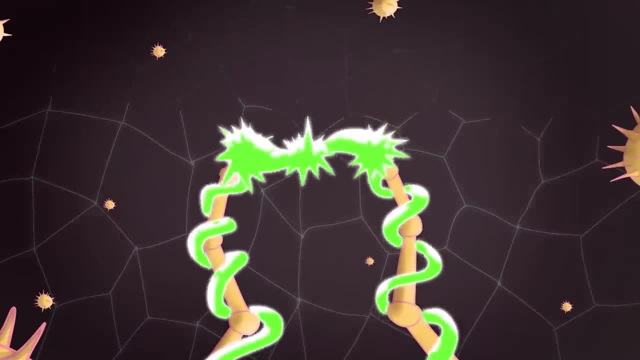 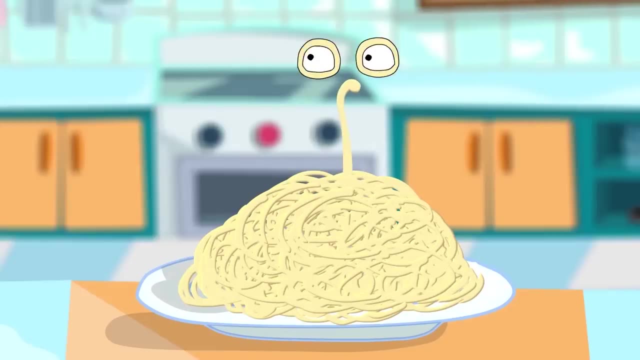 So we can make a warm drink. All right, immediately, Let's pour this into our reach. Oh, and also a little bit of boiling water. Now to get more ingredients. I need some space. I'm gonna go get some more water. That's a little smell of immerse. 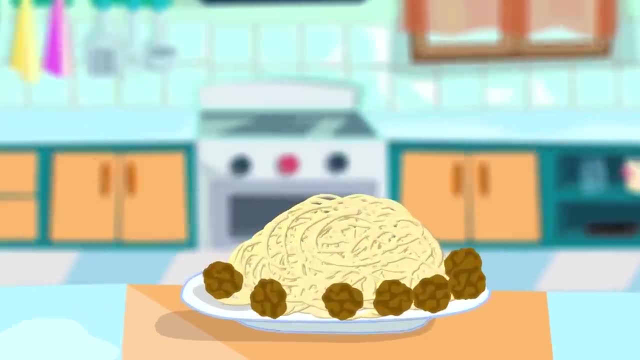 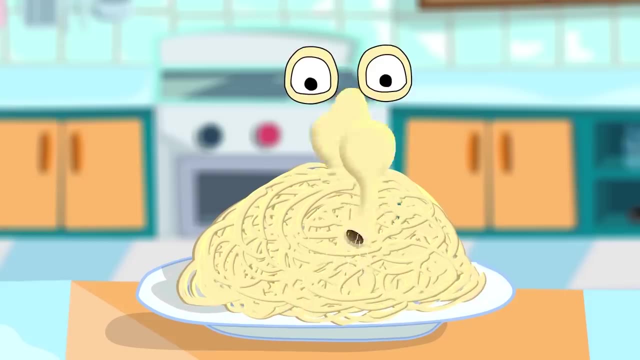 We're gonna need a little bit of this. I'm gonna go add some more salt. What do they call this? meh Shade? Yeah, I'm gonna add that right there. I'm gonna put these in the fridge for a couple of minutes. Okay, that's enough. 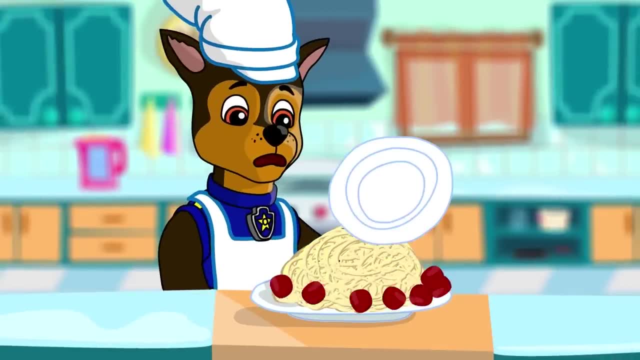 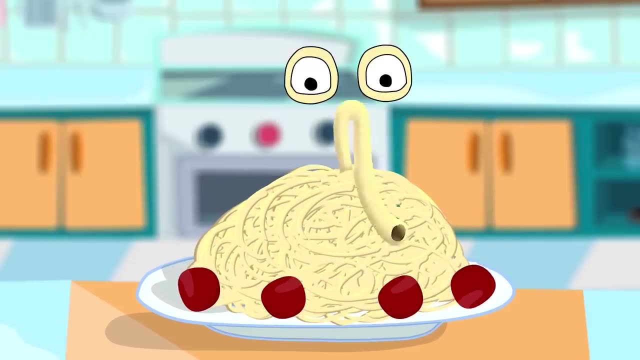 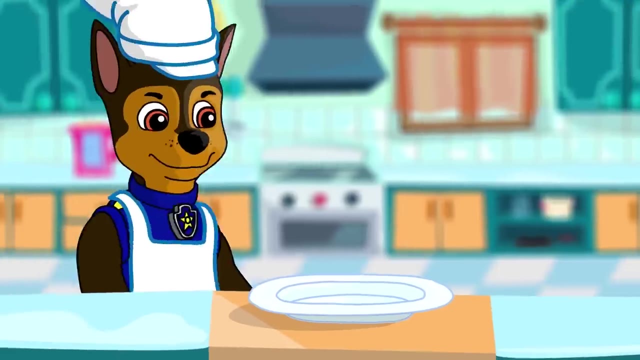 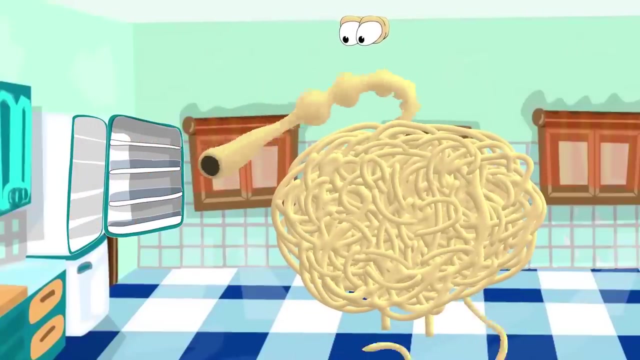 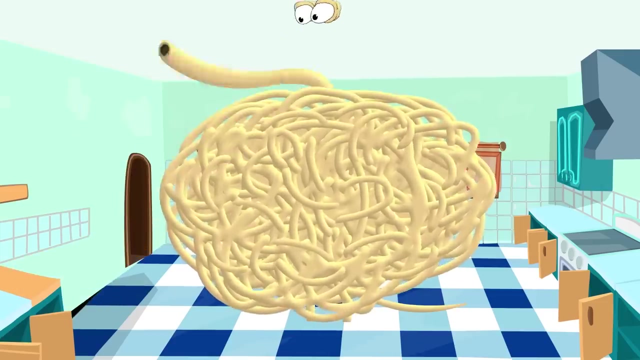 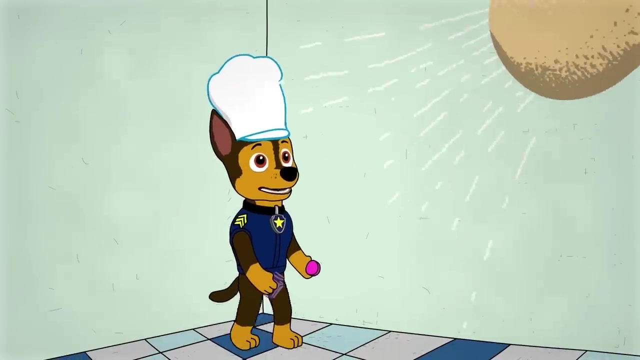 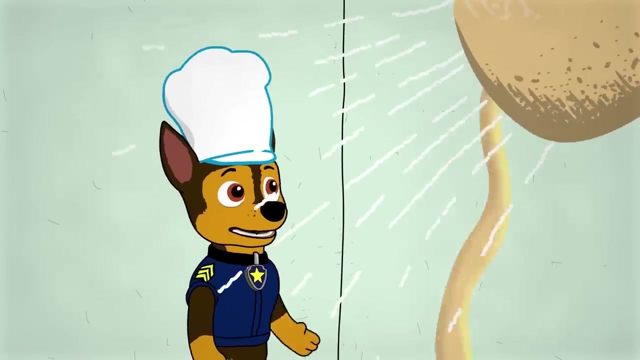 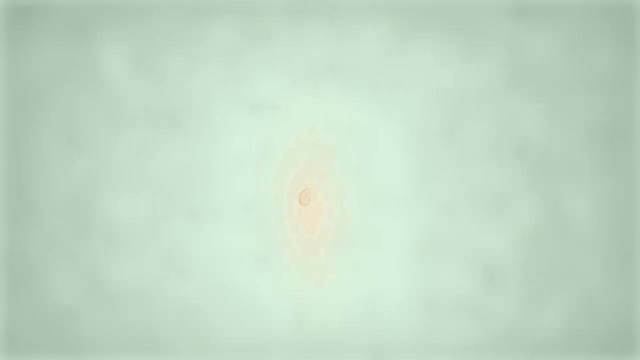 We're about ready to serve and I'm gonna want a drink. What in the world? Hey, where's the spaghetti? Oh Man, what am I gonna do? One plate of spaghetti done and done. Now it's Rubble's turn. He's gonna make. 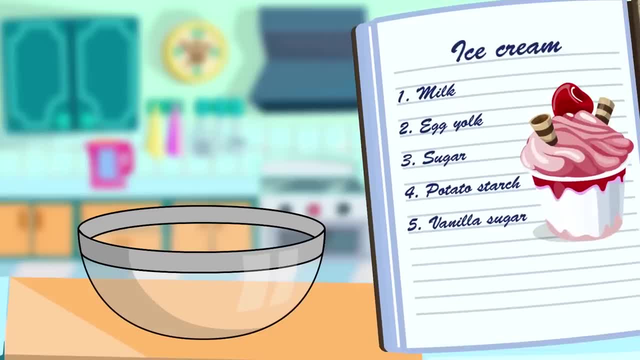 Ice cream for Everest. He'll need to pour milk in a bowl, Add some egg yolk, Some sugar to make it sweet, Some potato starch to give it consistency and Vanilla sugar to give it a special flavor. then mix it all together and put it in the freezer. 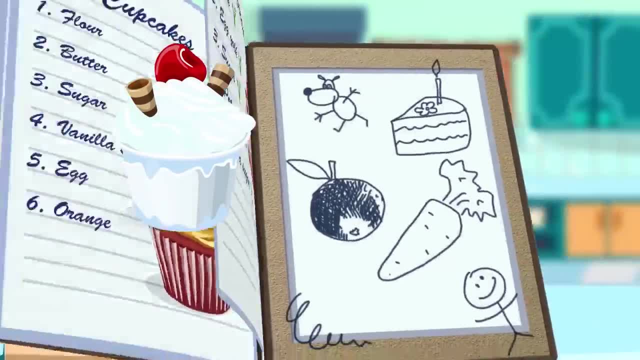 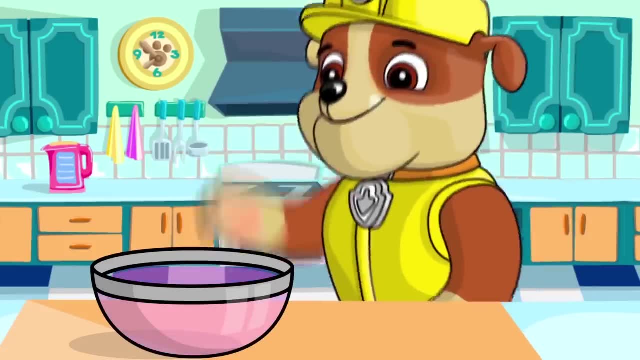 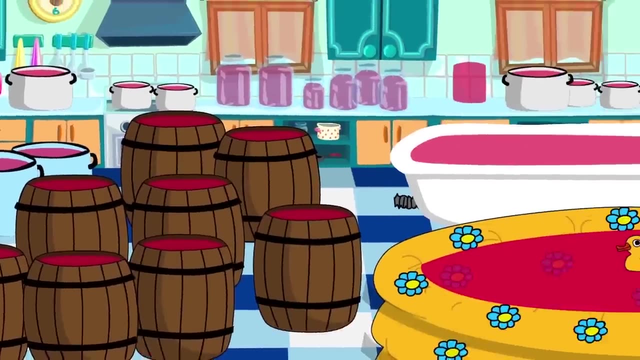 Then Rubble will have delicious ice cream. I'll do my own recipe. Are you sure? that's smart Rubble? Don't worry, I know what I'm doing. Mmm, I need more. I Hope that's enough. Oh man, how am I gonna freeze all this? 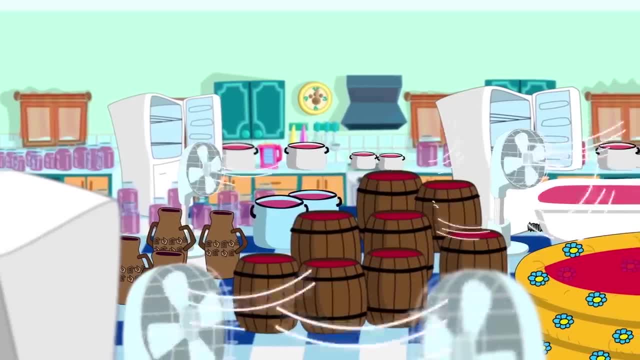 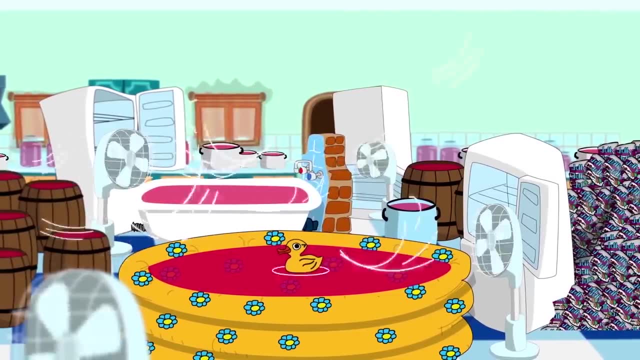 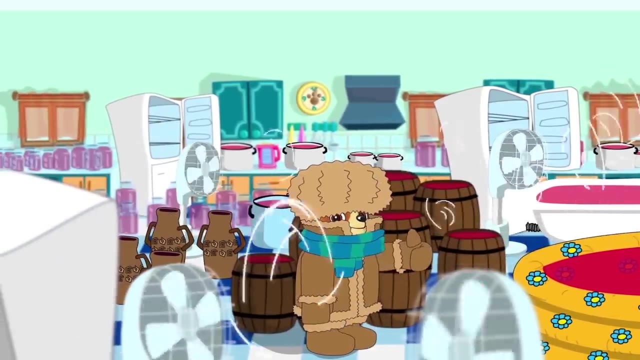 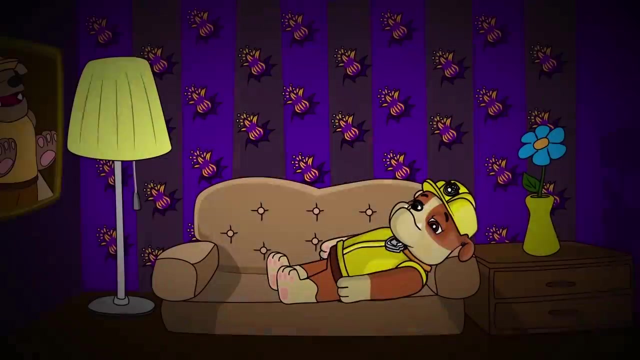 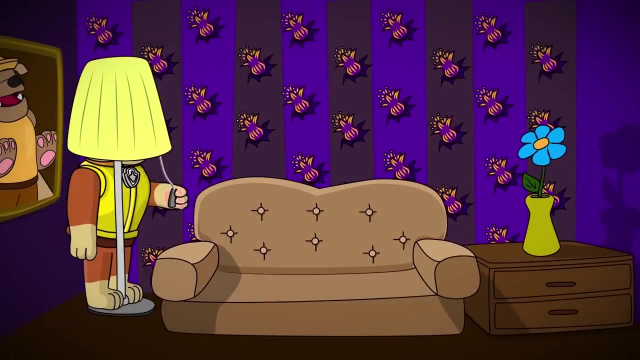 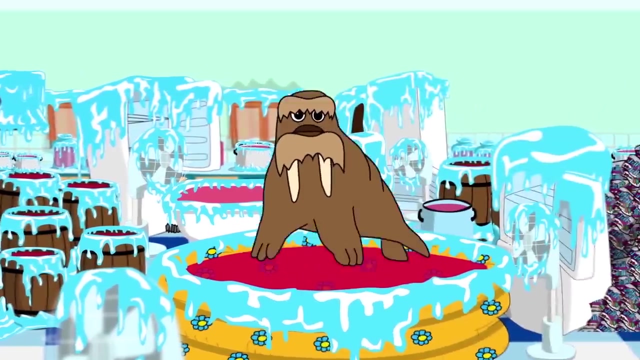 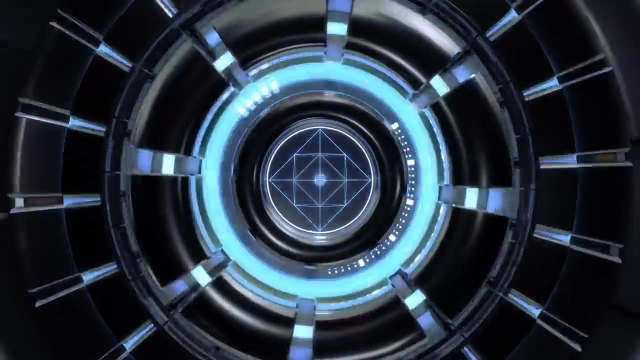 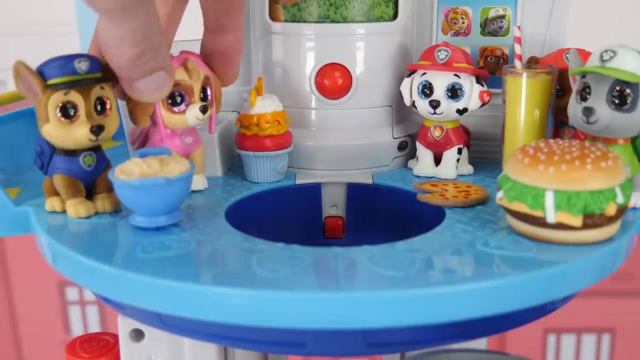 Hmm, Oh Boy, I'm a genius: 30 minutes, that's gonna take forever. This isn't so bad. one minute later, So bored, I know. Huh, Oh, Oh, Yummy, Everest will be here any minute. Did everyone finish cooking their food? Yep, and I had no problems at all. Yeah right, Marshal. Hey, where's Rubble? Wasn't he supposed to make ice cream? 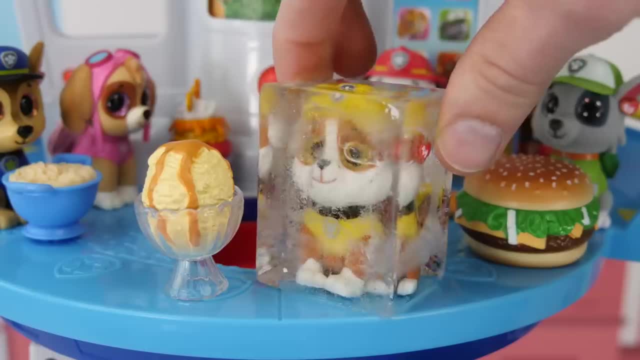 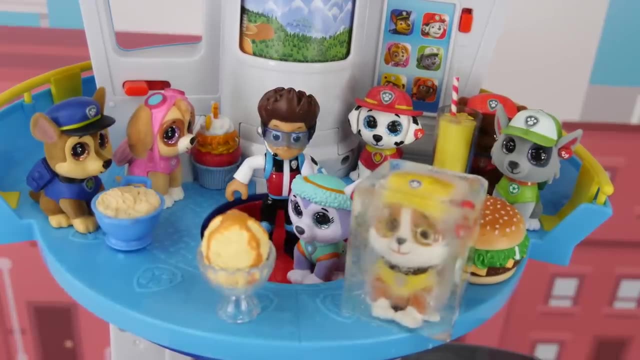 Um, Rubble. what happened? Oh Um, I just had a few minor difficulties. Guys, get ready, Everest is coming. Hi guys, how's it going? We heard you were coming, so we cooked you some food. Oh, that's really sweet of you guys. 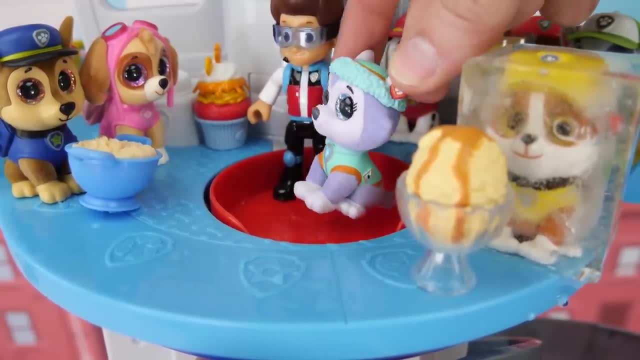 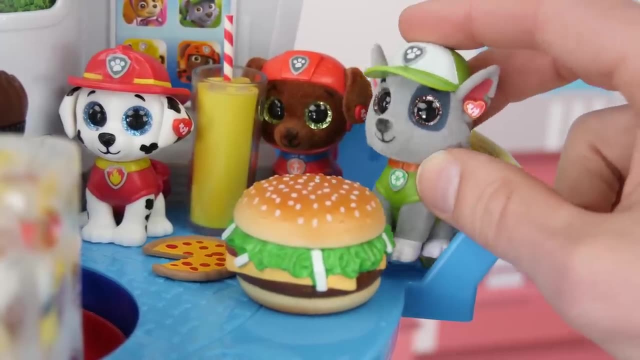 But Ryder and I stopped to get food on the way. Fool, oh. What are we gonna do with all this food? Well, I don't know about you guys, but I love leftovers. more importantly, What are we gonna do about me? I'm still frozen in this ice block. 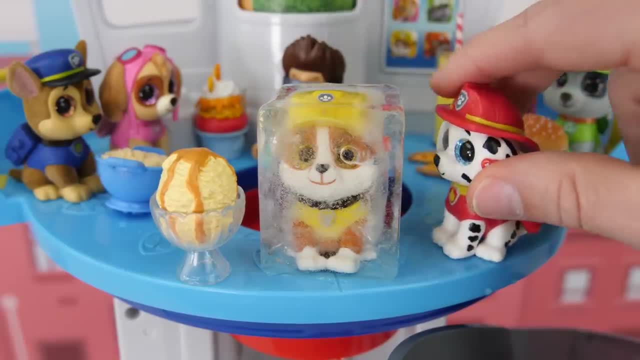 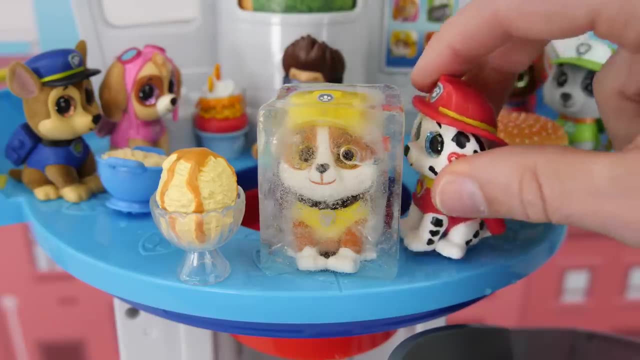 Don't worry, rubble, I got you covered. Mmm, you're tasty Yeah.